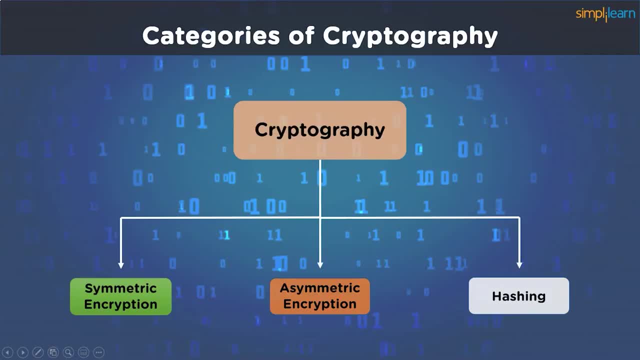 Meet Ann Ann wanted to look for a decent discount on the latest iPhone. Meet Ann Ann wanted to look for a decent discount on the latest iPhone. If you find this video interesting, make sure to give it a thumbs up before moving ahead. 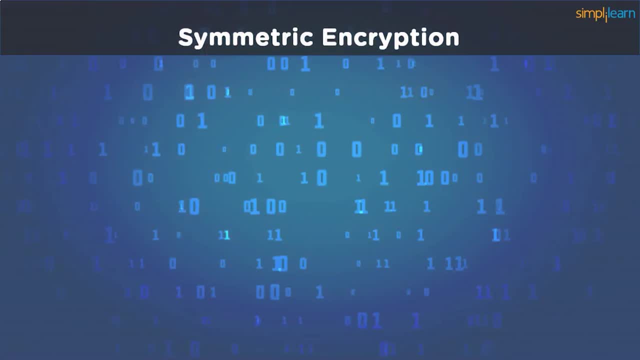 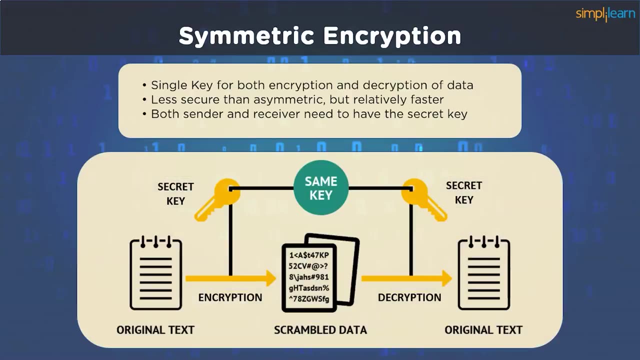 Let's look at symmetric encryption first. Symmetric encryption uses a single key for both the encryption and decryption of data. It is comparatively less secure than asymmetric encryption, but much faster. It is a compromise that has to be embraced in order to deliver data as fast as possible. 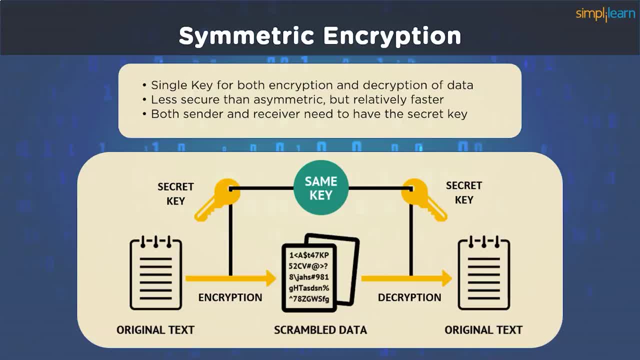 without leaving information completely vulnerable. This type of encryption is used when data rests on servers and identifies personnel for payment applications and services. The potential drawback with symmetric encryption is that both the sender and receiver need to have the same secret key and it should be kept hidden at all times. 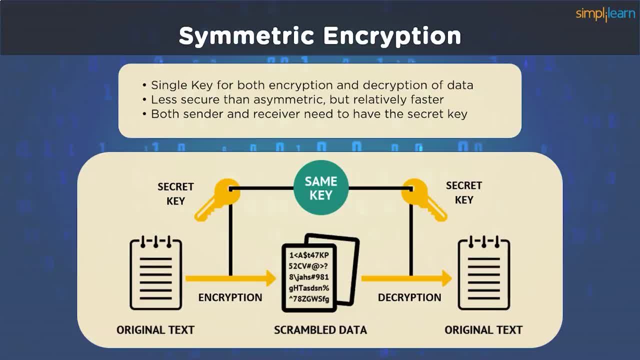 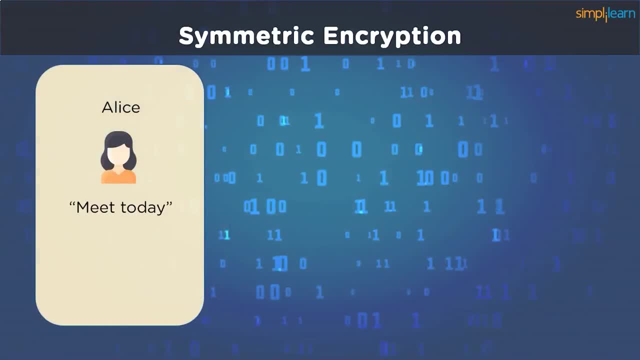 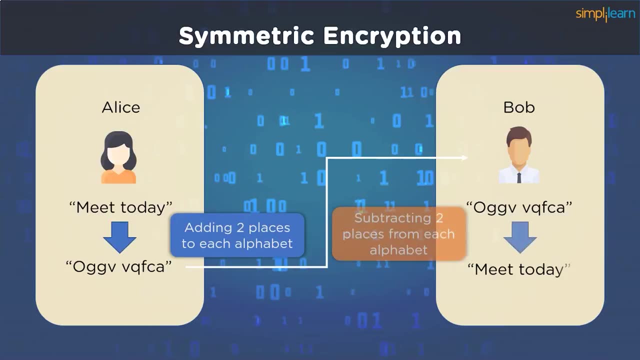 Caesar cipher and enigma machine are both symmetric encryption examples that we will look into further. For example, if Alice wants to send a message to Bob, she can apply a substitution cipher or a shift cipher, But Bob must be aware of the same key itself so he can decrypt it when he finds it necessary. 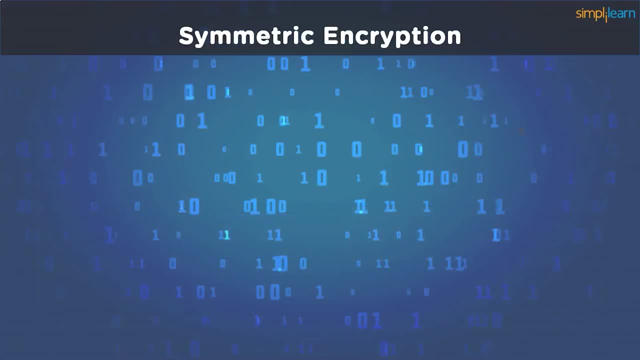 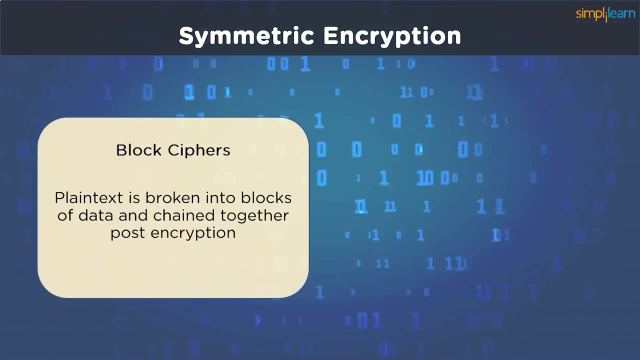 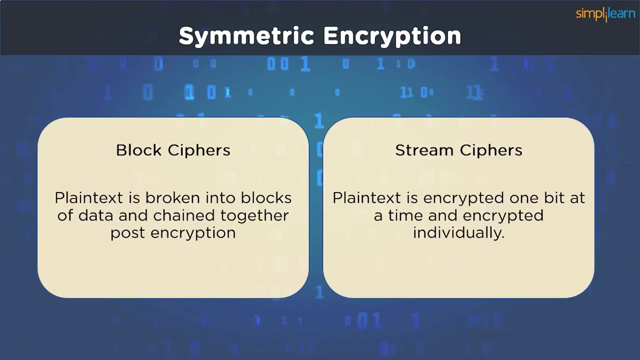 to read the entire message. Symmetric encryption uses one of the two types of ciphers: stream ciphers and block ciphers. Block ciphers break the plain text into blocks of fixed size and use the key to convert it into ciphertext. Stream ciphers convert the plain text into ciphertext one bit at a time, instead of resorting. 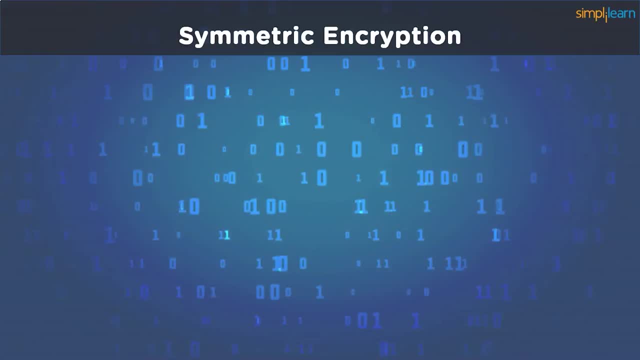 to breaking them up into blocks. In today's world, the most widely used symmetric encryption algorithm is AES-256. that stands for Advanced Encryption Standard, which has a key size of 256-bit, with 128-bit and 196-bit key sizes also being available. 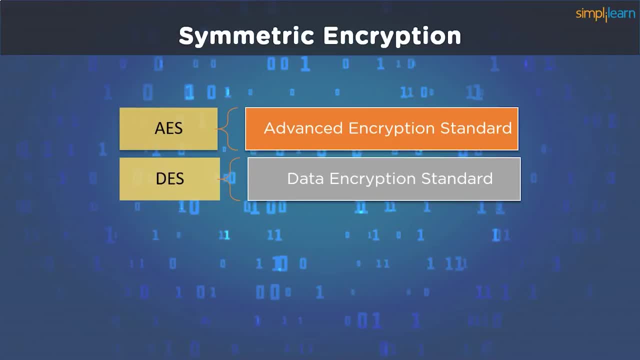 Other primitive algorithms like the Data Encryption Standard, the Triple Data Encryption Standard and Blowfish have all fallen out of favor due to the rise of AES. AES-256 is the most widely used symmetric encryption algorithm. AES chops up the data into blocks and performs 10 plus rounds of obscuring and substituting. 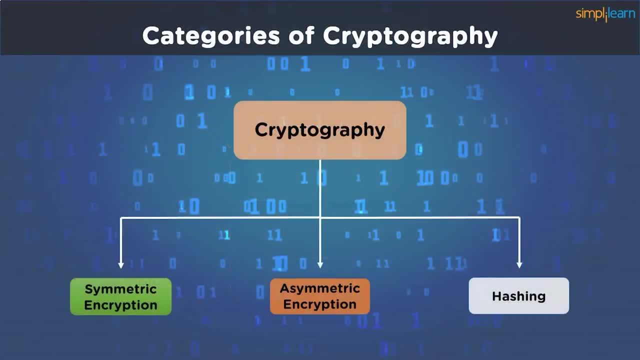 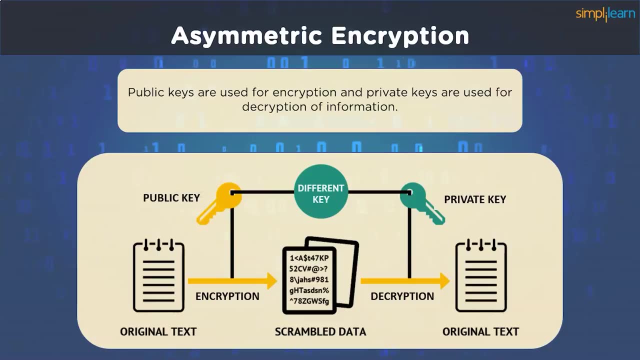 the message to make it unreadable. Asymmetric encryption, on the other hand, has a double whammy at its disposal. There are two different keys at play here, a public key and a private key. The public key is used to encrypt information pre-transit, and a private key is used to decrypt. 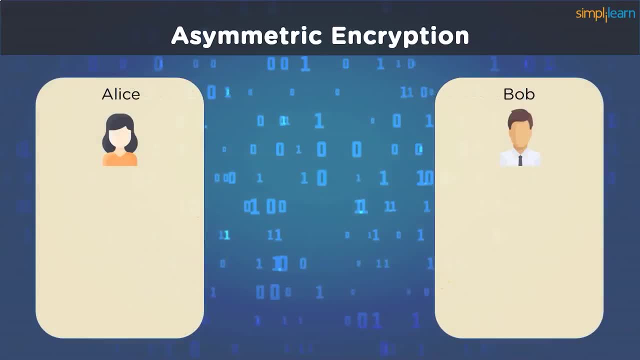 the information post-transit. If Alice wants to communicate with Bob using AES-256, the public key is used to decrypt the information post-transit. If Alice wants to communicate with Bob using asymmetric encryption, she encrypts the message using Bob's public key. 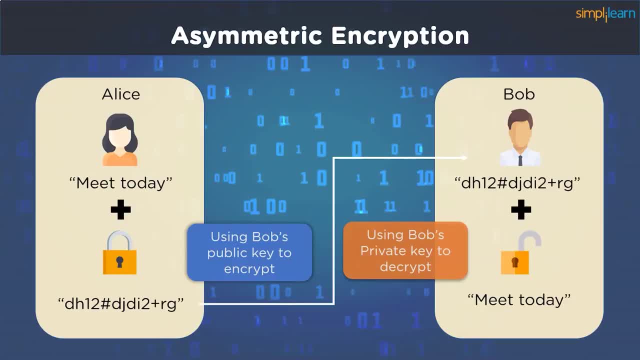 After receiving the message, Bob uses his own private key to decrypt the data. This way, nobody can intercept the message in between transmissions and there is no need for any secure key exchange for this to work, since the encryption is done with the public key and the decryption is done with the private key that no one except Bob has access to. 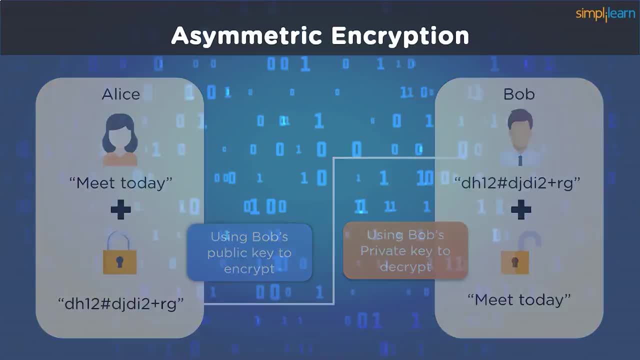 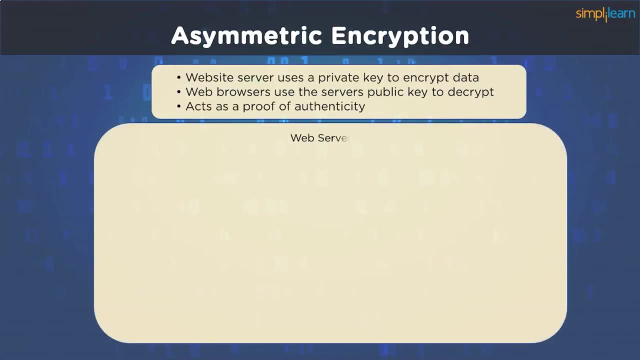 Both the keys are necessary to read the full message. There is also a reverse encryption Reverse scenario where we can use the private key for encryption and the public key for decryption. A server can sign non-confidential information using its private key and anyone who has its. 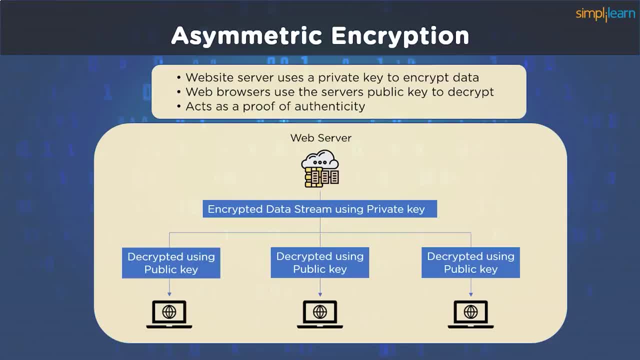 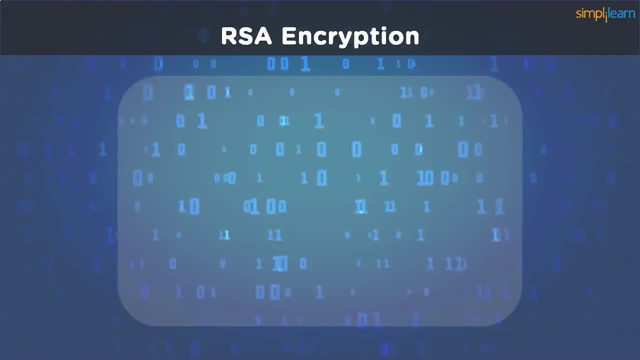 public key can decrypt the message. This mechanism also proves that the sender is authenticated and there is no problem with the origin of the information. RSA encryption is the most widely used asymmetric encryption standard. It is named after its founders, Rivest Shamir and Mahatma Gandhi. 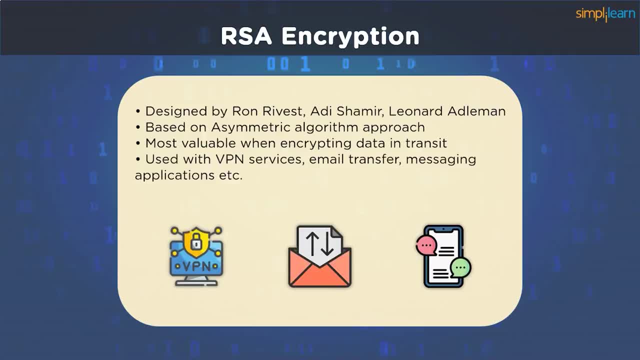 In recent years. RSA encryption is the most widely used asymmetric encryption standard. It is named after its founders, Rivest Shamir and Mahatma Gandhi and Edelman, and it uses block ciphers that separate the data into blocks and obscure the 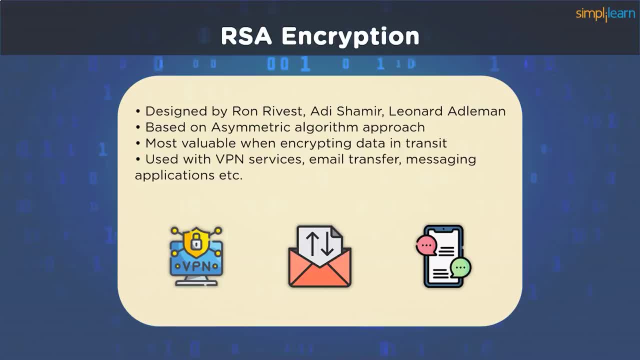 information, Widely considered the most secure form of encryption, albeit relatively slower than AES. it is widely used in web browsing, secure identification, VPNs, emails and chat applications. With so much hanging on the keys secrecy, there must be a way to transmit the keys without others. 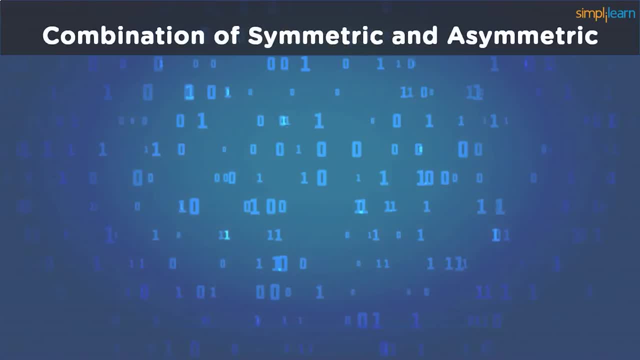 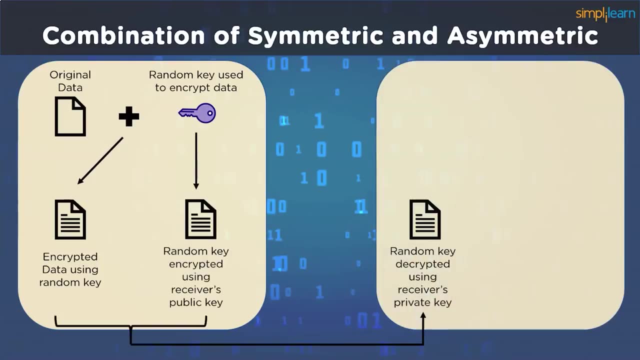 reading our private data. Many systems use a combination of symmetric encryption and asymmetric encryption to bolster security and match speed at the same time. Since asymmetric encryption takes longer to decrypt large amounts of data, the full information is encrypted using a single key that is symmetric encryption. That single key is then transmitted to the receiver using 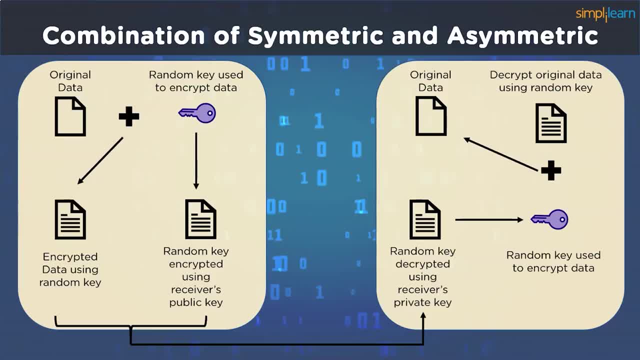 asymmetric encryption, so you don't have to compromise either way. Another route is using the Diffie-Hellman key exchange- Diffie-Hellman key exchange, which relies on a one-way function and is much tougher to break into. The third variant of cryptography is termed as hashing. 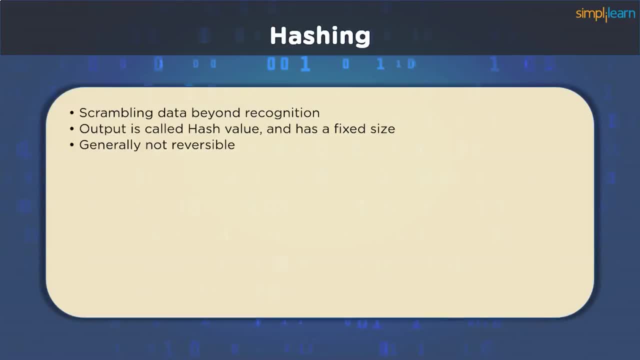 Hashing is the process of scrambling a piece of data beyond recognition. It gives an output of fixed size, which is known as the hash value of the original data, or just hash in general, The calculations that do the job of messing up the data collection form, the hash function. 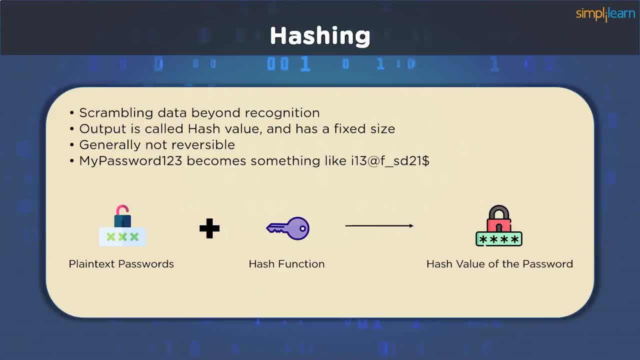 They are generally not reversible without resilient brute force mechanisms and are very helpful when storing data on website servers that need not be stored in plain text. For example, many websites store your account passwords in a hashed format so that not even the administrator can read your credentials When a user tries to log. 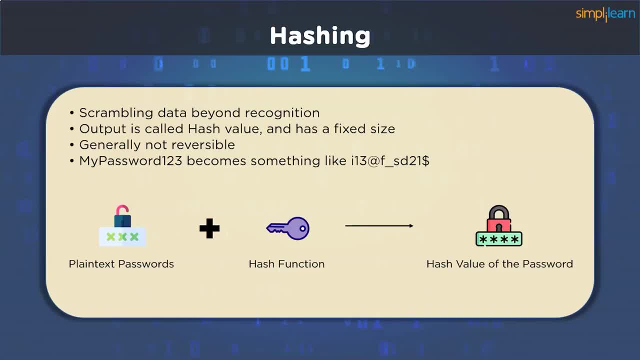 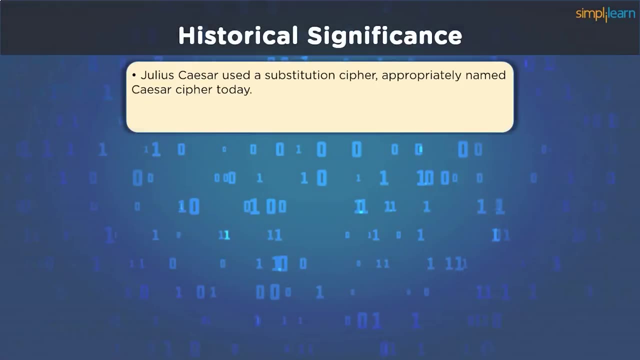 in, they can compare the entered password's hash value with the hash value that is already stored on the servers for authentication. since the function will always return the same value for the same input, Cryptography has been in practice for centuries. Julius Caesar used a substitution shift to 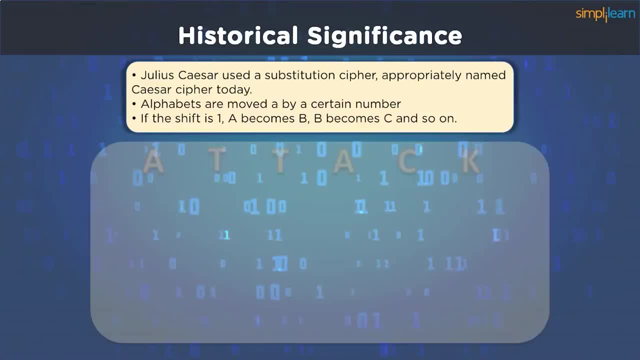 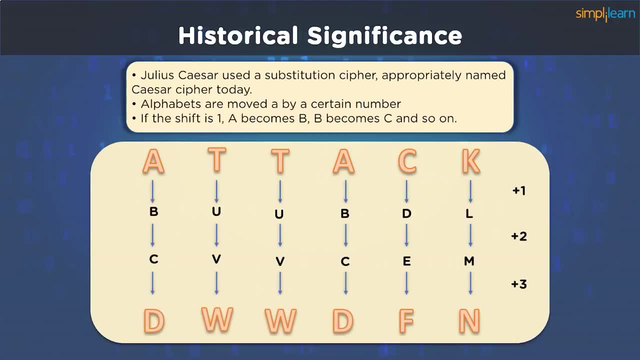 move alphabets a certain number of spaces beyond their place in the alphabet table. A spy can't decipher the original message at first glance. For example, if he wanted to pass confidential information to his armies and decides to use the substitution shift of plus two, A becomes C, B becomes D and so on. The word attack when passed through. 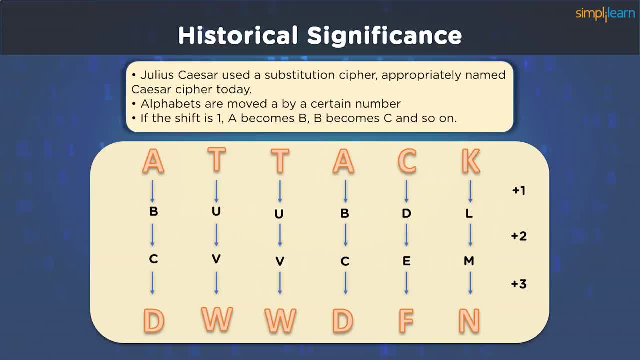 a substitution shift of plus three is used as an example. The word attack, when passed to a substitution shift of plus three, is used as an example. The word attack, when passed through a substitution shift of plus three, becomes D-W-W-D-E-F-N or. 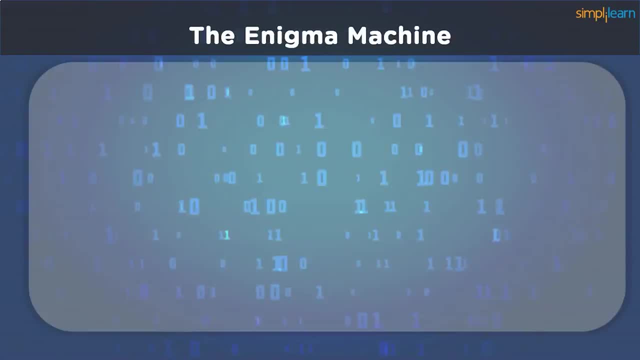 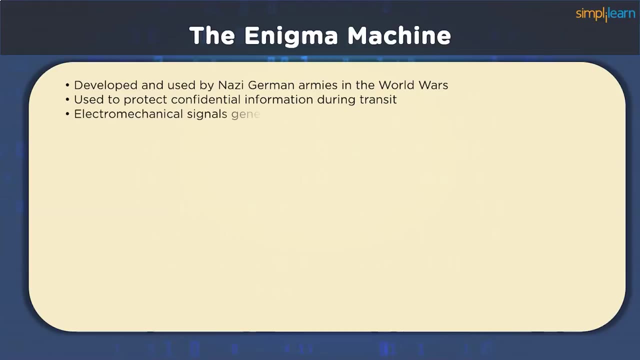 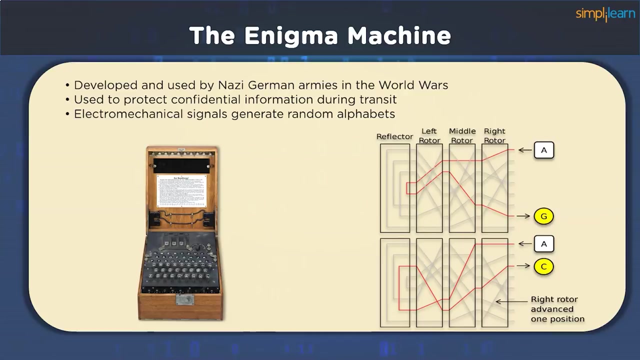 the Caesar Cipher, The enigma, is probably the most famous cryptographic cipher device used in ancient history. It was used by the Nazi German armies in the world wars. They were used to protect confidential political, military and administrative information, and it consisted of three or more rotars that. 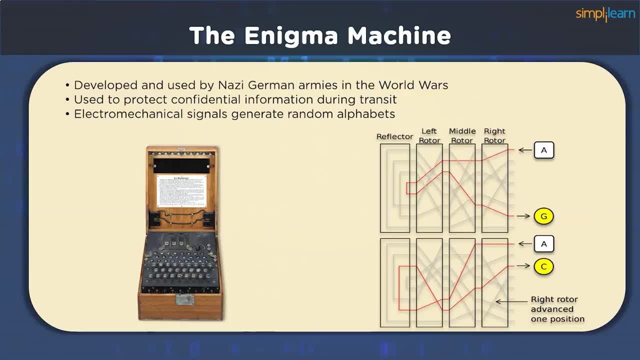 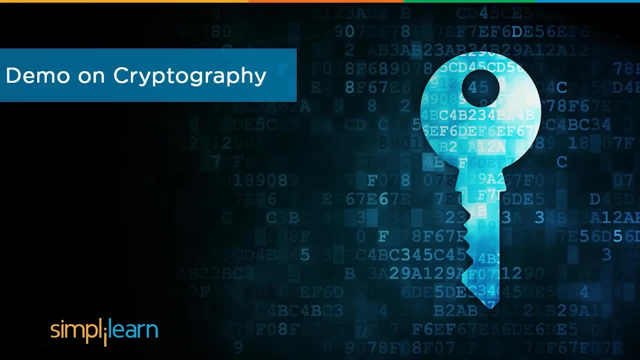 Let's scramble the original message, depending on the machine's state at that time. The decryption is similar, but it needs both machines to stay in the same state before passing the ciphertext so that we receive the same plain text message. Let's take a look at how our data is protected while we browse the internet, thanks to cryptography. 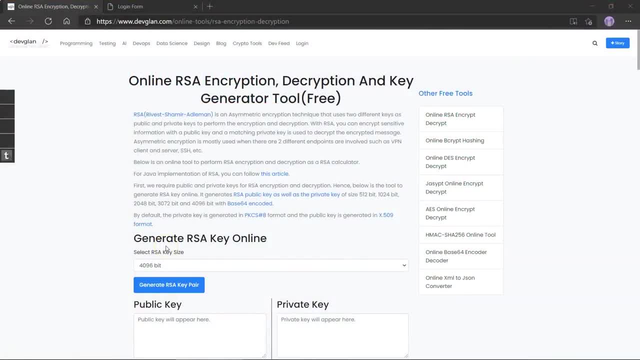 Here we have a web-based tool that will help us understand the process of RSA encryption. We see the entire workflow, from selecting the key size to be used until the decryption of the ciphertext in order to get the plain text back. As we already know, RSA encryption algorithm falls under the umbrella of asymmetry key. 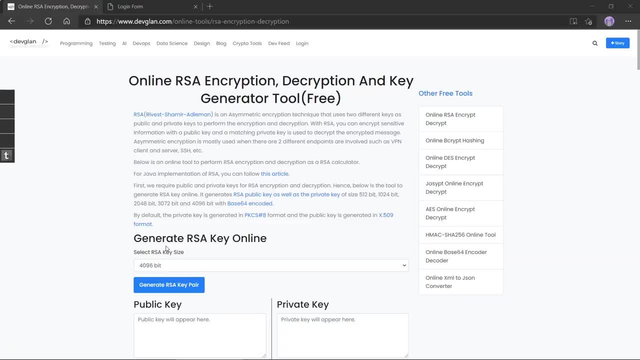 cryptography. That basically implies that we have two keys at play here, a public key and a private key. Typically, the public key is used by the sender to encrypt the message and the private key is used by the receiver to decrypt the message. There are some occasions when this allocation is reversed, and we will have a look at them. 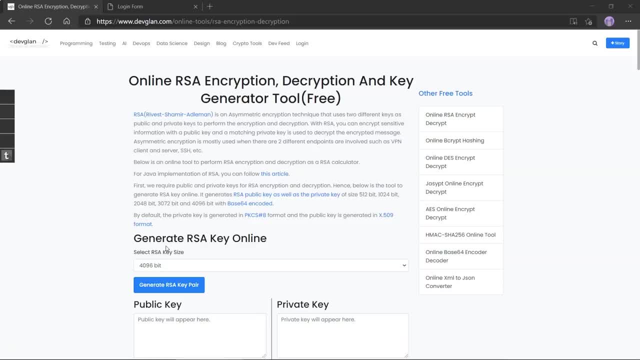 as well In RSA, we have the choice of key size. We can select any key from a 512-bit to 1024-bit, all the way up to a 4096-bit key. The longer the key length, the more complex the encryption process becomes, and thereby 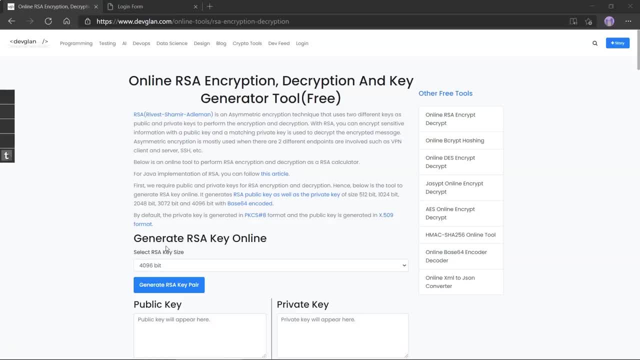 strengthening the ciphertext, Although with added security. more complex functions take longer to perform the same operations on similar sizes of data. We have to keep a balance between both speed and strength, because the strongest encryption algorithms are of no use. Let's take a 1024-bit key over here. 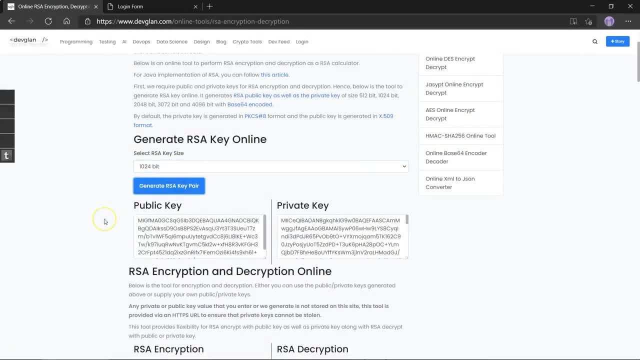 Now we need to generate the keys. This generation is done by functions that operate on passphrases. The tool we are using right now generates these pseudo-random keys to be used in this explanation. Once we generate the keys, you can see the public key is rather smaller than the private. 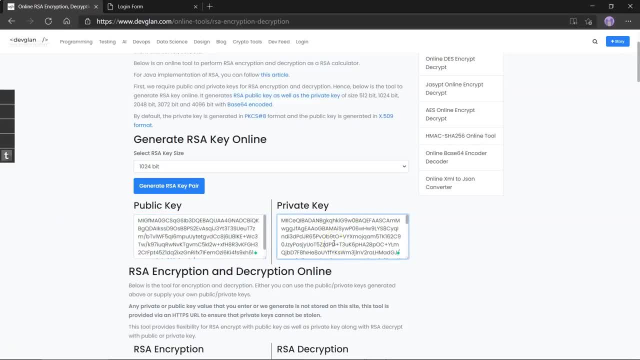 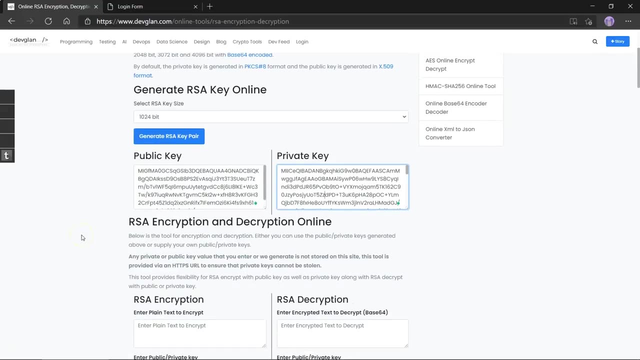 key, which is almost always the case. These two keys are mathematically linked with each other. They cannot be substituted with any other key and, in order to encrypt the original message or decrypt the ciphertext, this pair must be kept together. The public key is then sent to the sender and the receiver keeps the private key with. 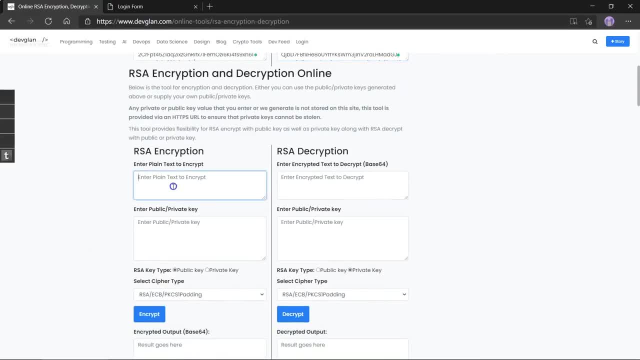 himself. In this scenario, let's try and encrypt a word. simply learn. We have to select if the key being used for encryption is either private or public, since that affects the process of scrambling the information, Since we are using the public key over here. 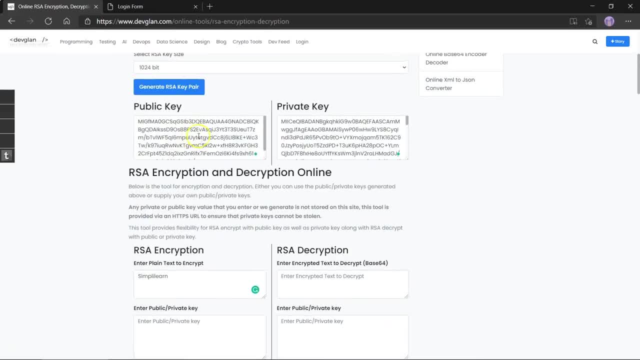 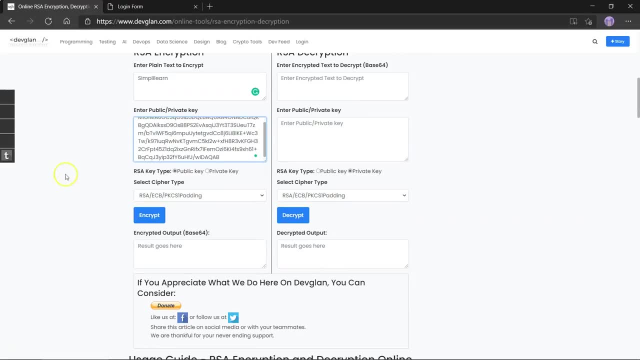 Let's select the same and copy it and paste over here. The cipher we are using right now is plain RSA. There are some modified ciphers with their own pros and cons that can also be used, provided we use it on a regular basis and depending on the use case as well. 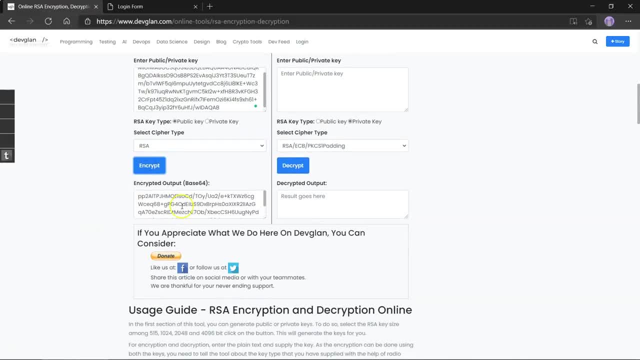 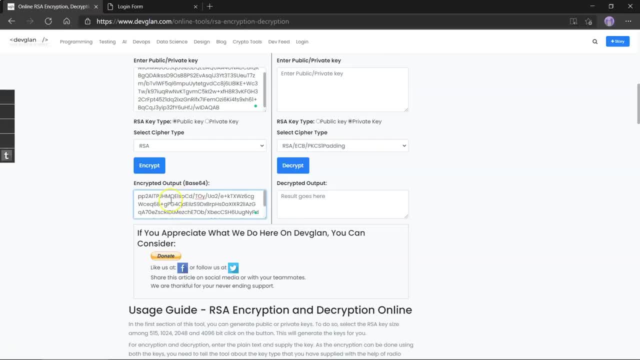 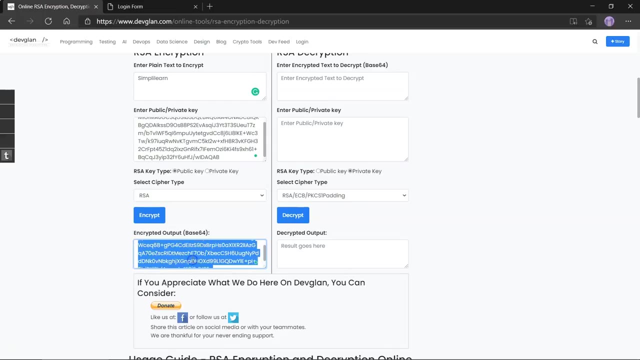 The pseudo-random generating functions are kept together. These are created in such a way that a single character change in the plaintext will trigger a completely different ciphertext. This is a security feature to strengthen the process from brute force methods. Now that we are done with the encryption process, let's take a look at the decryption part. 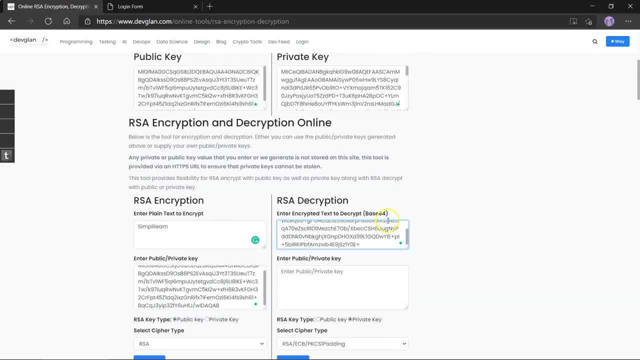 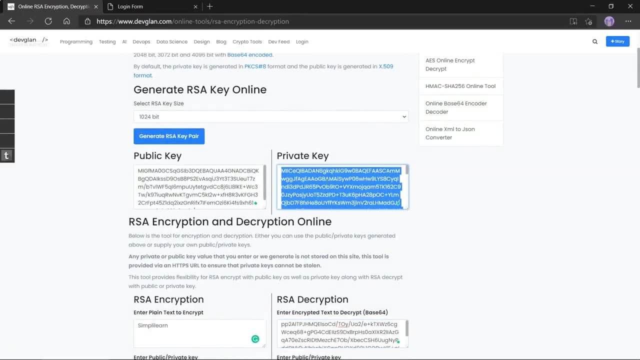 The receiver gets this ciphertext from the sender with no other key or supplement. He or she must already possess the private key generated from the same pair. no other key can be used to decrypt the message. since they are mathematically linked. We paste the. 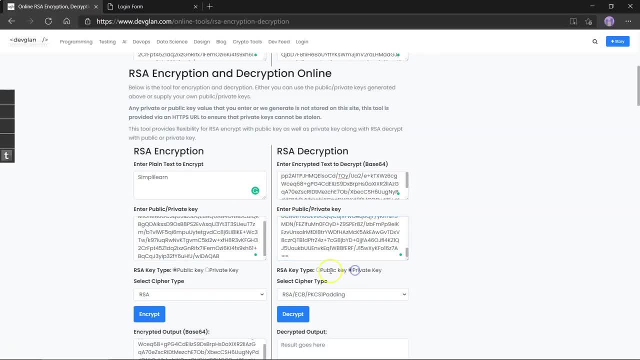 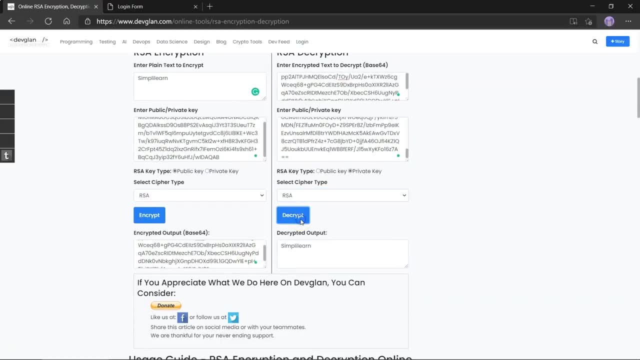 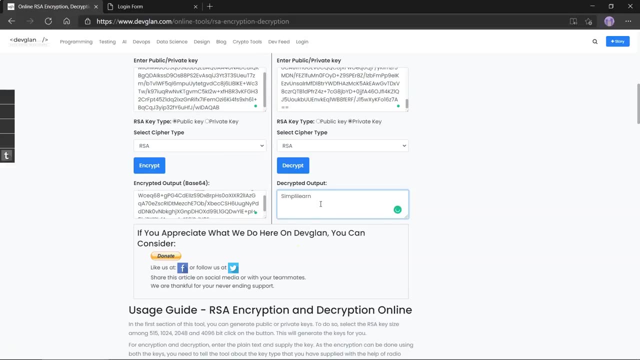 private key here and select the same. The cipher must always so be the same used during the encryption process. Once we click decrypt, you can see the original plain text we had decided to encrypt. This sums up the entire process of RSA encryption and decryption. 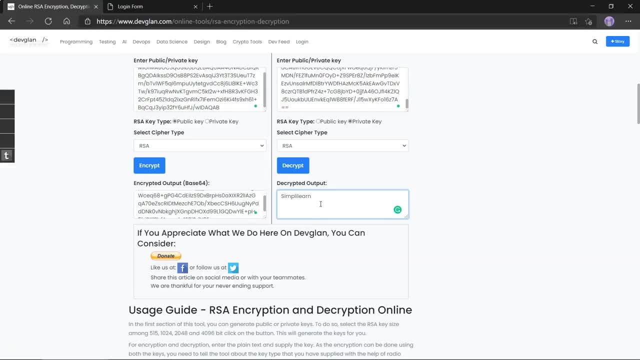 Now some people use it the other way round. We also have the option of using the private key to encrypt information and the public key to decrypt it. This is done mostly to validate the origin of the message, Since the keys only work in pairs if a different. 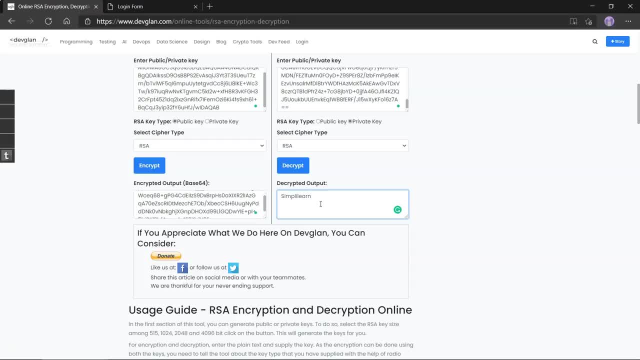 private key is used to encrypt the message, the public key cannot decrypt it. Conversely, if the public key is able to decrypt the message, it must have been encrypted with the right private key and hence the rightful owner. Here we just have to take the private key. 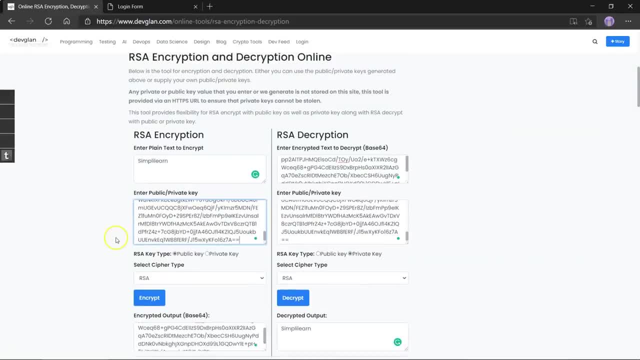 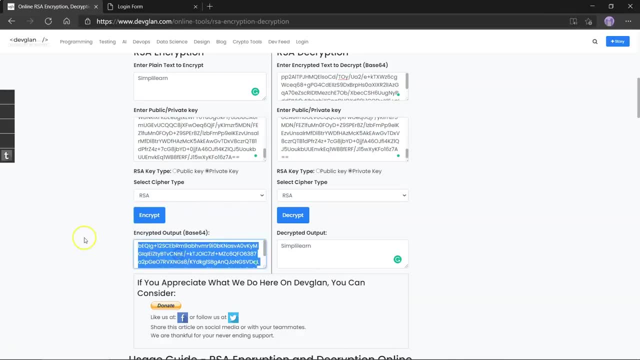 and use that to encrypt the plain text and select the same in this checkbox. You can see we have generated a completely new cipher text. This cipher text will be sent to the receiver and this time we will use the public key for decryption. Let's 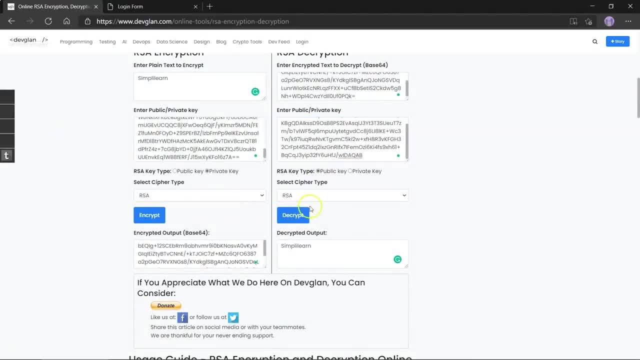 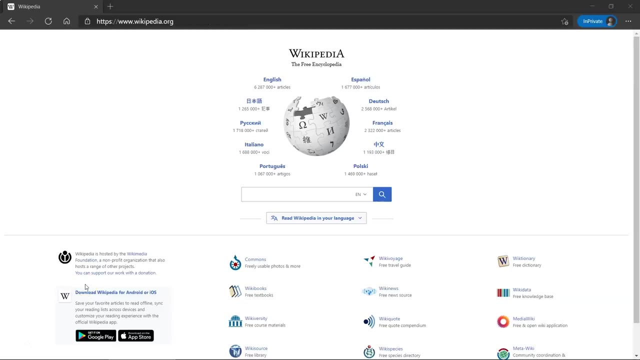 select the correct checkbox and decrypt, and we still get the same output. Now let's take a look at practical example of encryption in the real world. We all use the internet on a daily basis and many are aware of the implications of encryption in the real world. 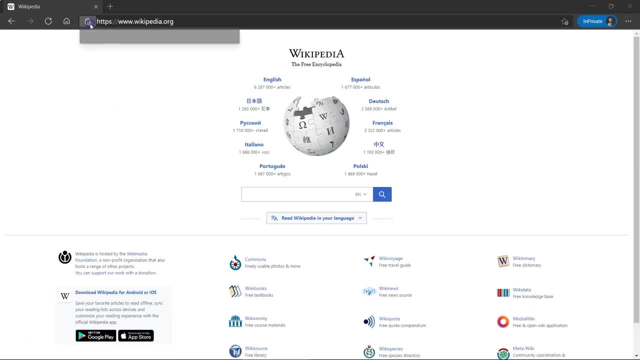 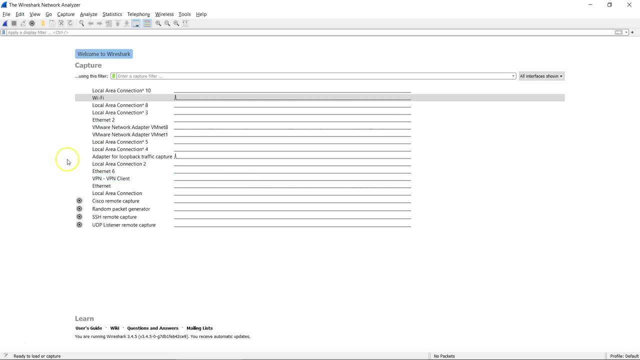 of using unsafe websites. Let's take a look at Wikipedia here: Pretty standard HTTPS website where the H stands for secured. Let's take a look at how it secures the data. Wireshark is the world's foremost and most widely used network protocol analyzer. It lets you see what's happening on your network at. 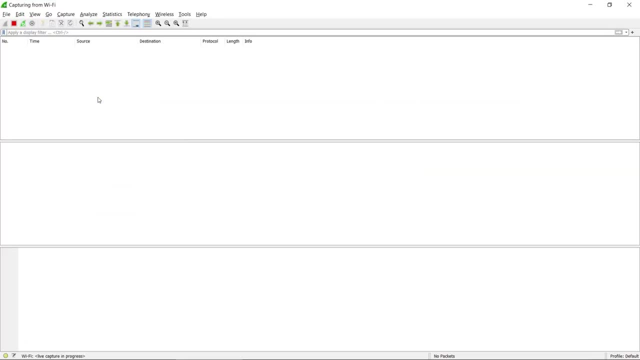 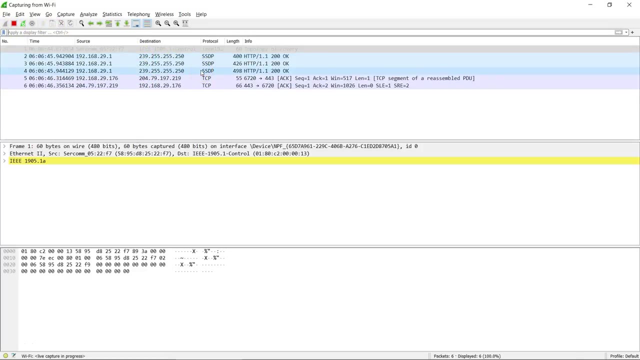 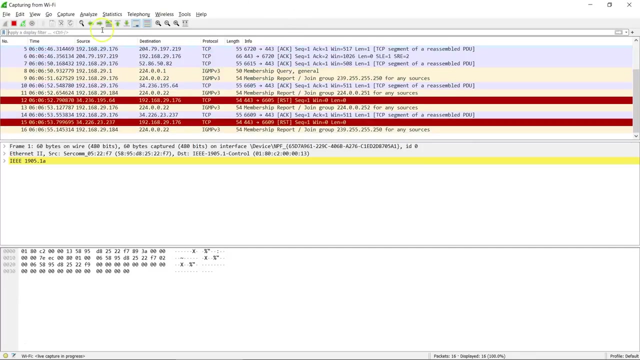 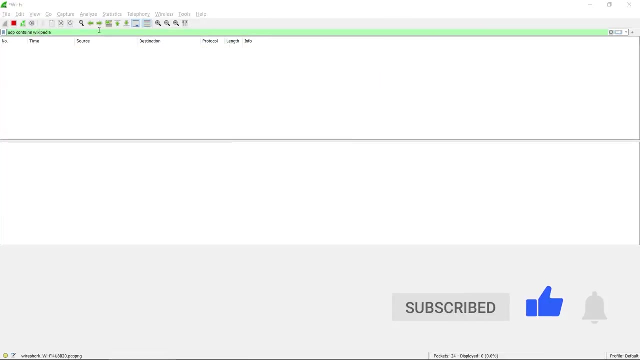 a microscopic level, and we are going to use the software to see the traffic that is leaving a machine and to understand how vulnerable it is. Since there are many applications running in this machine, let's apply a filter that will only show us the results related to Wikipedia. Let's search for something. 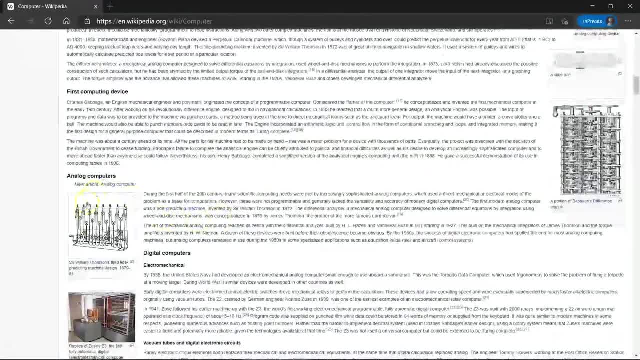 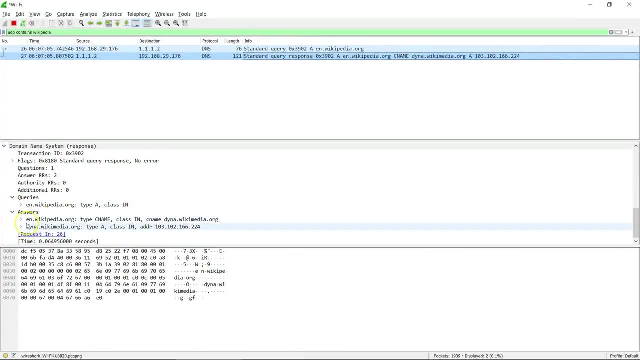 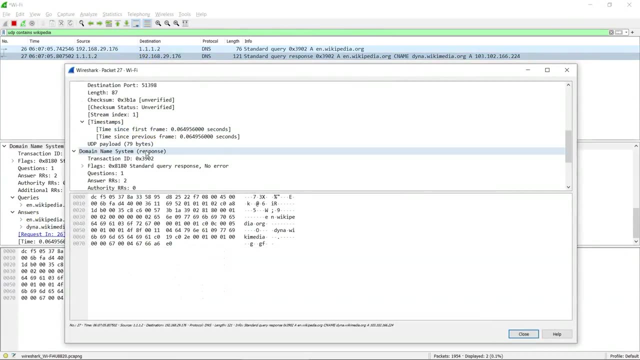 that we can navigate the website with. Okay, once we get into it a little, You can see some of the requests being populated over here. Let's take a look at the specific request. These are the data packets that basically transport the data from our machine to the internet and vice versa. As you can see, there's a bunch of 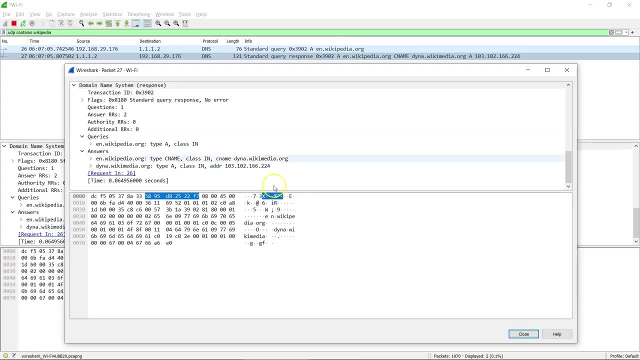 gibberish data here that doesn't really reveal anything that we searched or watched. Similarly, user-secured websites function the same way, and it is very difficult, if at all possible, to snoop on user data this way. To put this in perspective, let's take a look at another. 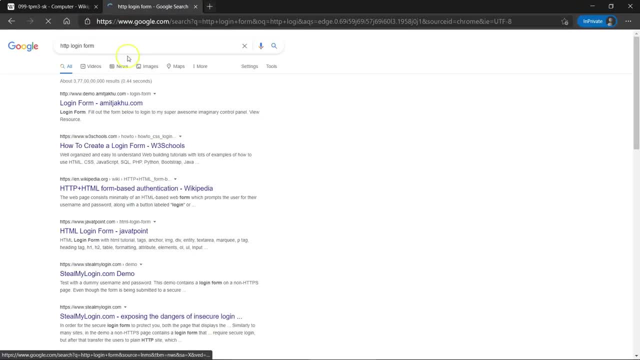 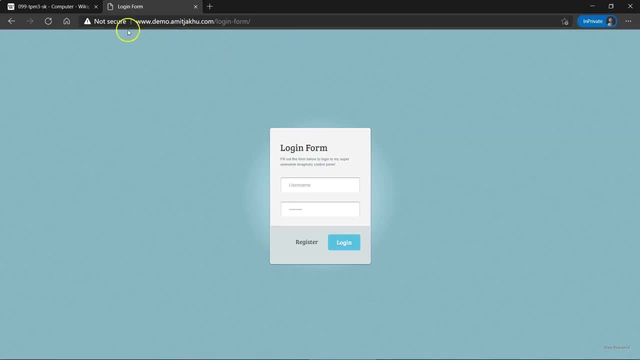 website, which is a HTTP webpage. This has no encryption enabled from the server end, which makes it vulnerable to attacks. There is a login form here which needs legitimate user credit. Let's enter a random pair of credentials in order to grant access. Let's enter a random.